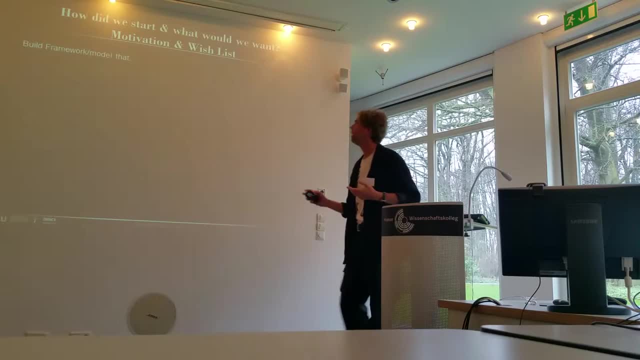 So we started this at the Max Planck Institute and we wanted to really build a framework that helps us understand what is going on, because of potential causes of spatial orientation problems, especially in virtual reality, where people get lost so much. So we wanted to know what is going on there. 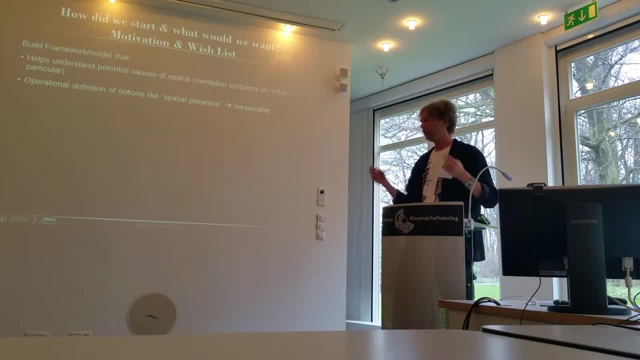 Also, we're just back on a train from a presence conference and we were quite frustrated with the lack of any clear operational definitions of what that really means and how to measure it. So we asked ourselves questions like: well, is there anything you really need spatial presence for? 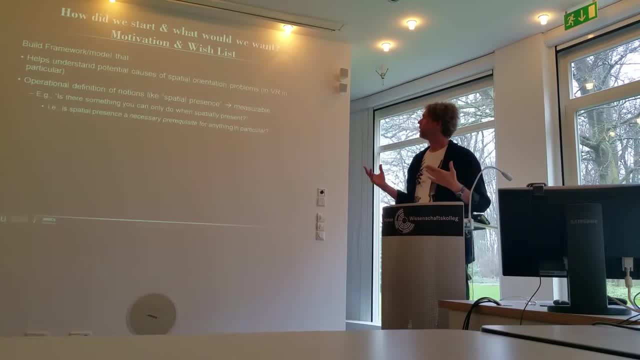 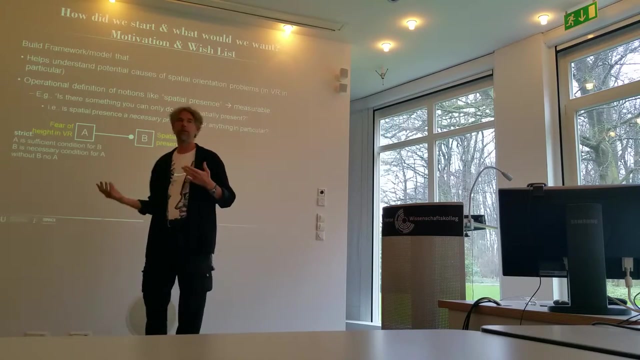 So basically, is spatial presence a necessary prerequisite for anything in particular, And so this idea of necessary prerequisite is basically what is used in logic quite a bit. So one example we thought of was: well, you probably wouldn't have any fear of height in virtual reality. 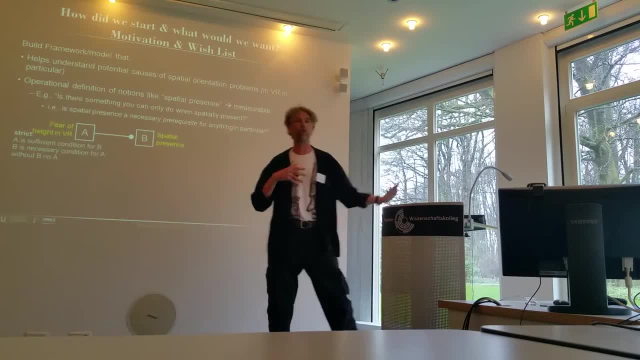 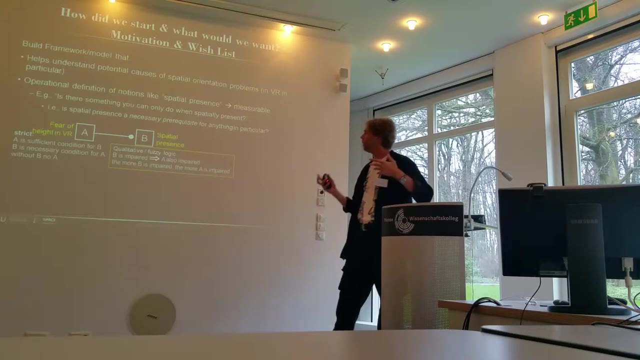 unless you really are fully immersed and you're no longer aware of the physical environment. Otherwise you might not really encounter it. And because, while we're dealing with humans and not with American politics, it's not a binary thing, So we think more of fuzzy logic. 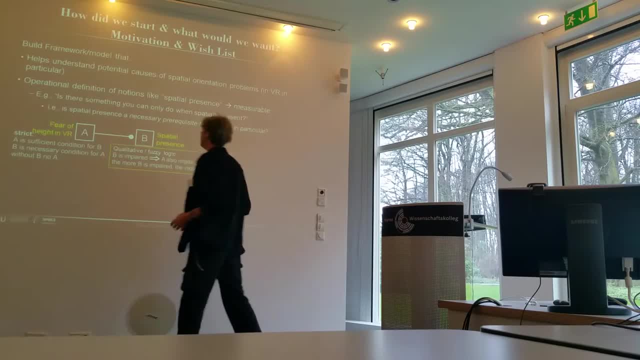 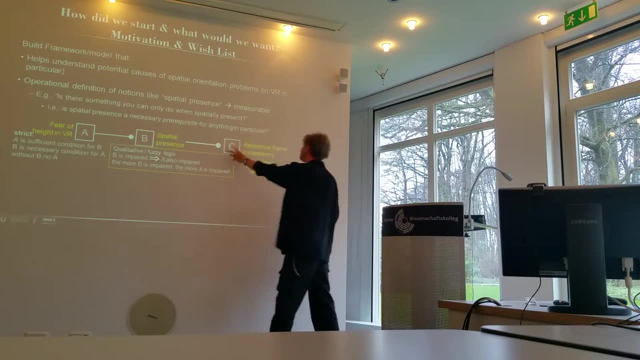 So basically, the more spatial presence is incurred, the more fear of height should also be inherent in virtual reality. And then we can kind of build up a logical chain. For example, we proposed that spatial presence implies that there's basically not much of a reference frame of conflict going on. 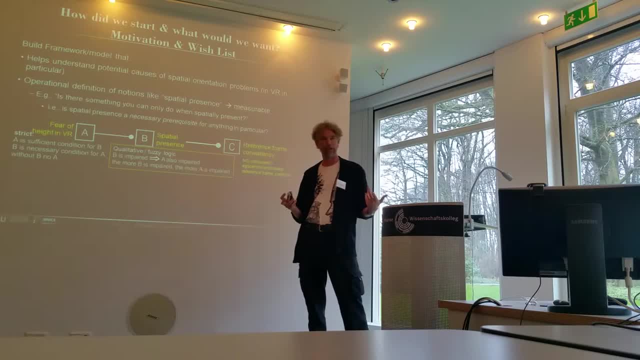 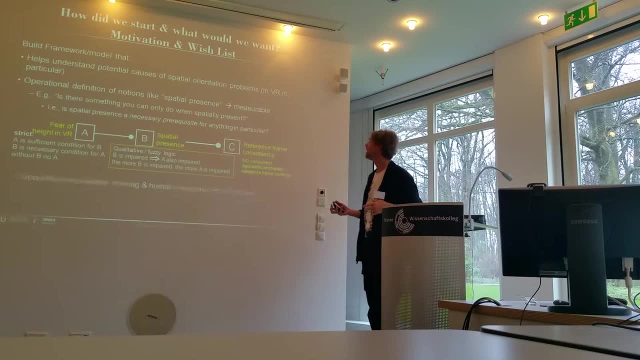 between what you're, for example, simulating and virtual reality and where you're physically at. So now I'm concurring egocentric reference frame conflicts with the ones that Marius might have mentioned. Also we wanted, given that we're in spatial cognition. 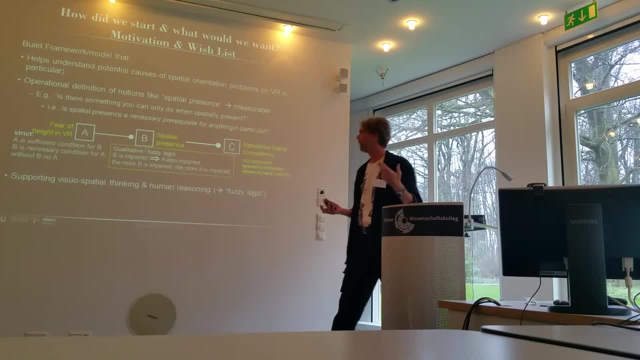 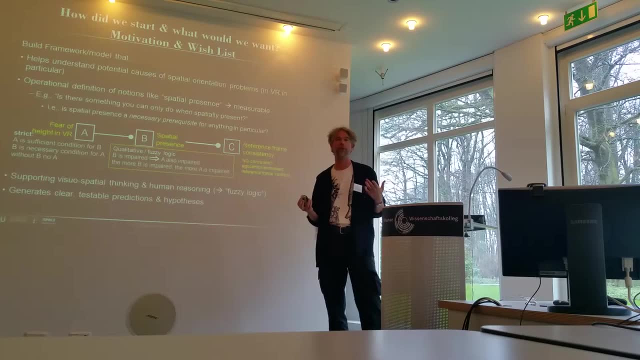 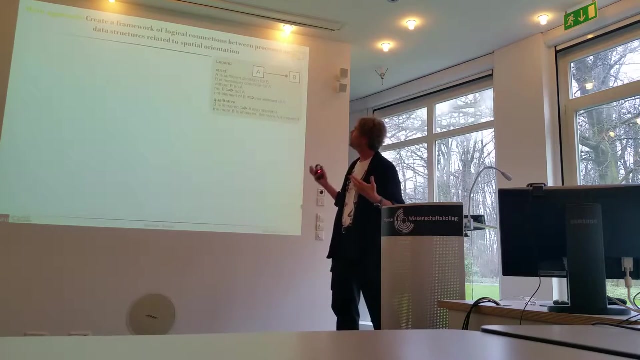 we wanted to build a tool or a visual representation that really facilitates, supports visual spatial thinking and human reasoning and also creates testable prediction hypotheses. You can see we were quite frustrated with the presence community at the time, So to do this we tried to create a framework of logical connections. 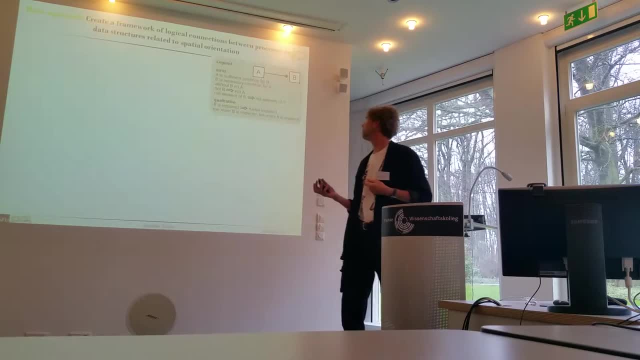 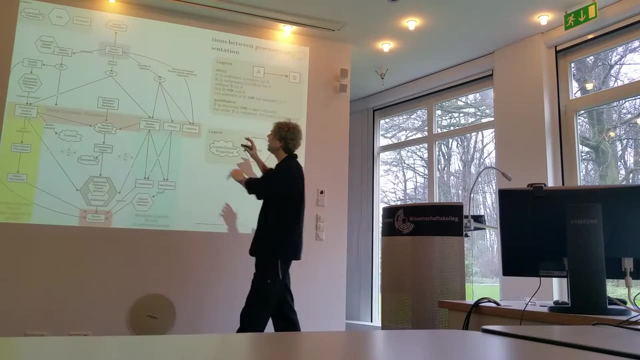 between processes and structures related to spatial orientation, distinguish between data, processes, goals in there, and came up with this kind of visual representation. I won't go through the whole thing. The main idea is, if you have some different spatial orientation at the top, 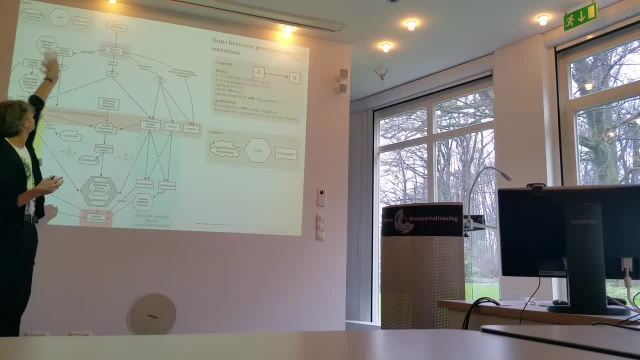 as the ultimate goal and you have different kinds of spatial behavior, so adaptable, learning-oriented. this is the main part I focused on. This is about more intuitive, quick orientations are based on spatial orientation. You can also have spatial updating processes. 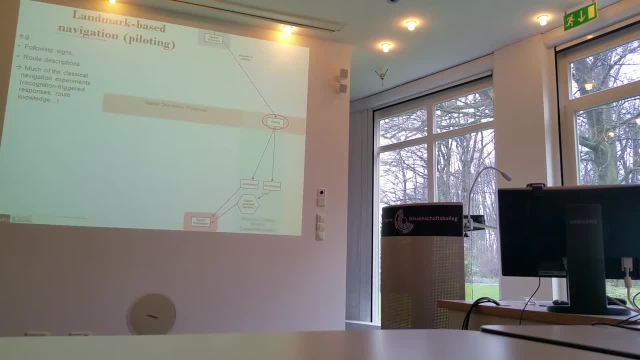 You can also have landmark-based accurate, precise navigation, things like that. So just as an example, so the whole landmark navigation branch here. so for piloting probably, for example, you necessarily need to be able to identify some kind of objects. 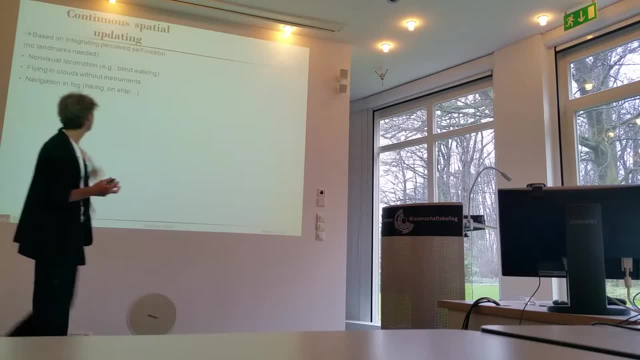 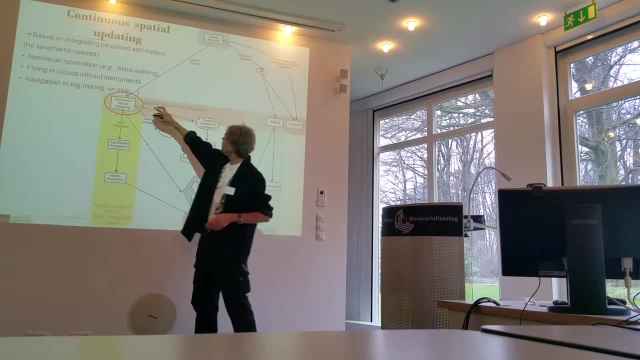 that you have in your landmark memory. You need to be able to vocalize them, Otherwise this just won't work For spatial updating. it's kind of similar This side. So in order to do continuous spatial updating, you obviously need to perceive self-motion. 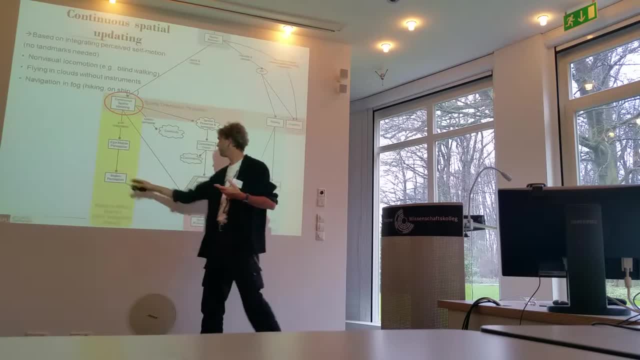 and then integrate this. For this to happen, you have to have some kind of motion perception. For this to happen, you have to have also spatial perception. But in addition there's other parts, For what we propose is that spatial presence at the neuron. 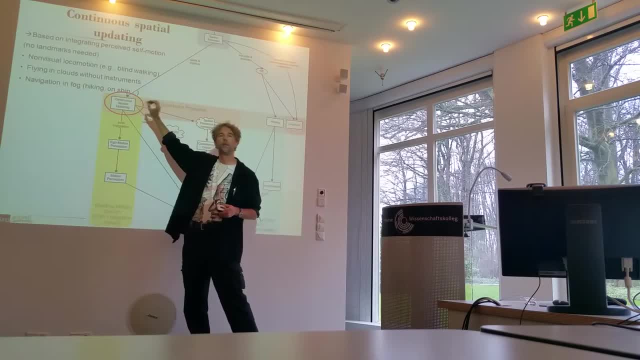 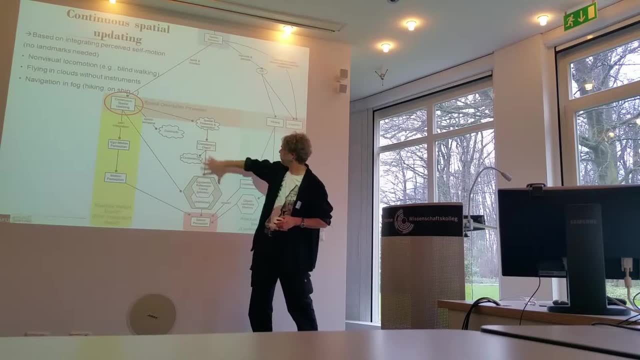 is a necessary prerequisite for you to really tap into these automatized low cognitive load processes like automatic spatial updating. Spatial updating will only happen if this kind of consistency check between concurrent reference frame gives a green light. basically, So it tells you there's a strong conflict between 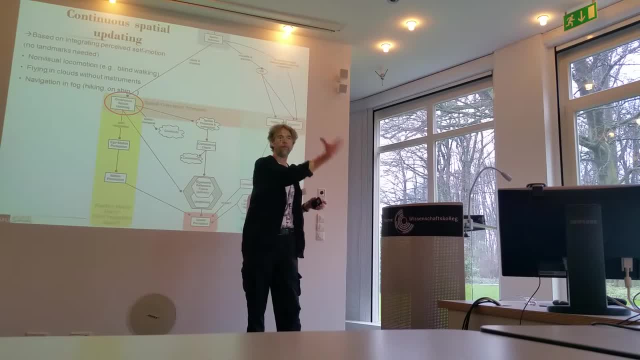 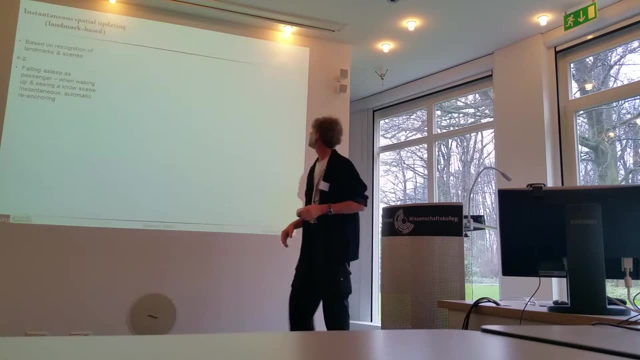 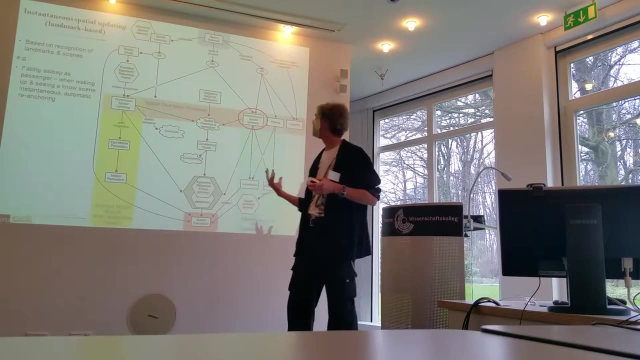 where you're physically at and what you're supposed to imagine and what virtual reality is doing, Then you won't be very present. This will interfere with continuous spatial updating And similar also with this instantaneous or instant-based spatial updating. What we mean by that is- let me give you an example- So if you fall asleep as a passenger in a car, you wake up, you recognize the space almost immediately. as soon as you recognize it, it kind of forcefully re-anchors you to that point And there's probably anything you can do about it. 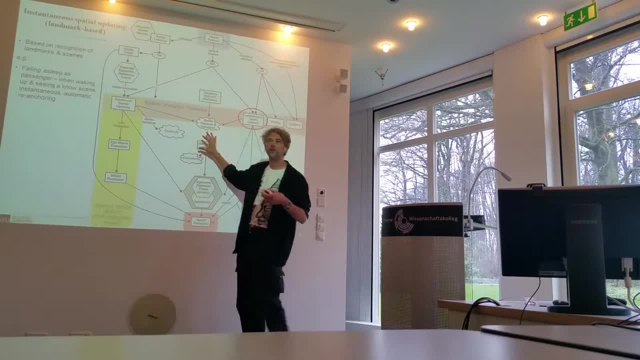 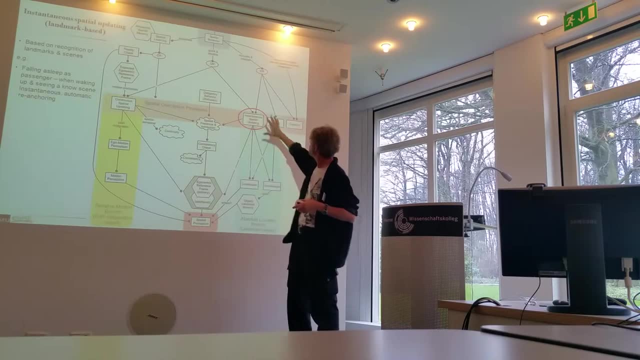 As soon as you recognize it. it's there Because there isn't much interference going on, because there wasn't really too much of prior spatial representation, And then virtual reality can have a similar thing, basically. So, with this kind of instant-based or instantaneous spatial updating, 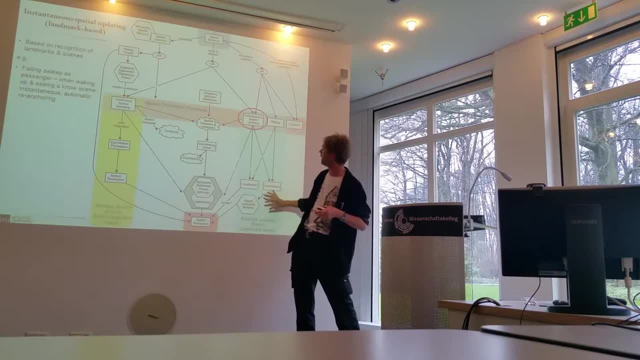 again, you have the localization graphs. you need to identify localized landmarks and you need to be spatially present. So I'd like to talk a little bit more about what is going on in this reference frame. So it's all kind of pictorial and iconic. 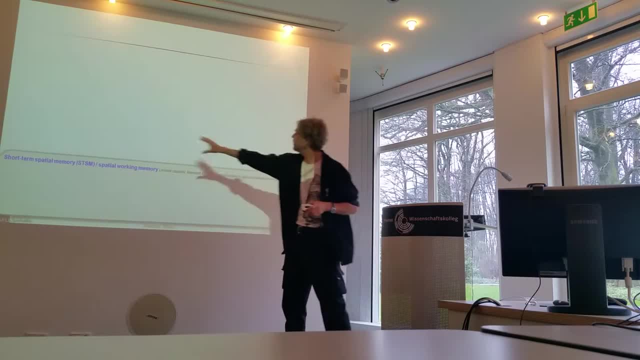 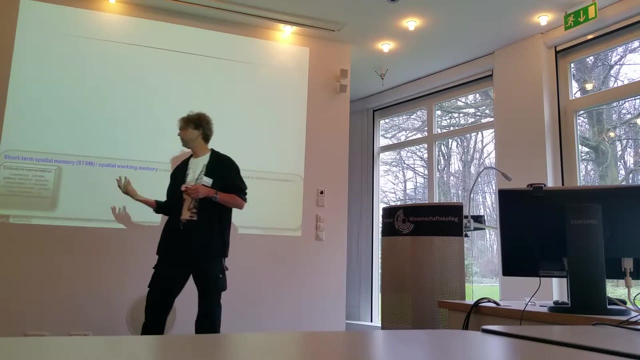 but I guess that's just closer to the way I think. So if this is kind of all boxed for short-term spatial memory or spatial networking memory, the little limited capacity transient representation, then we have some kind of embodied representation that could be the automatically activated sensory motor representation. 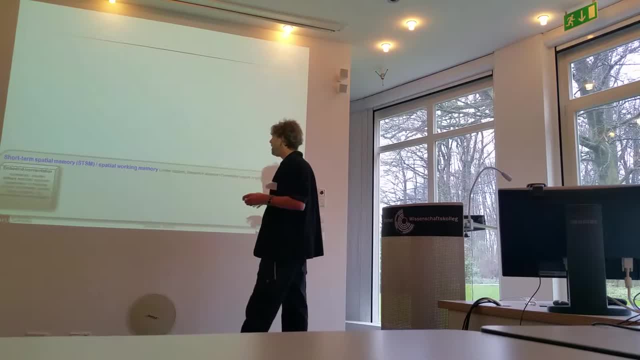 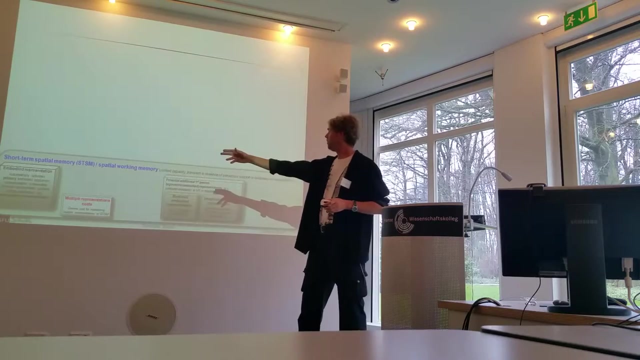 that especially Mariusz talked about in his experiment there. But you could have additional representations. This could be an imagined representation with an imagined task, or a mediated, embodied representation, like in virtual reality or other media. And, of course, if you deal with multiple representations, 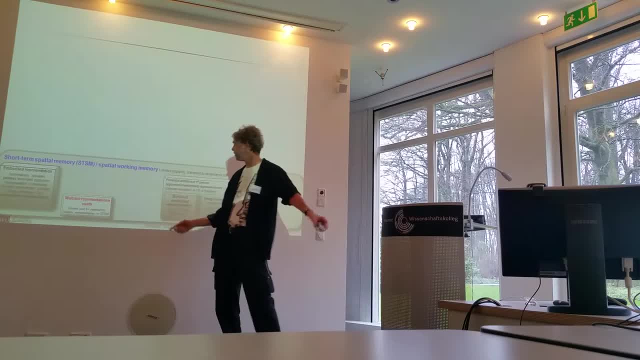 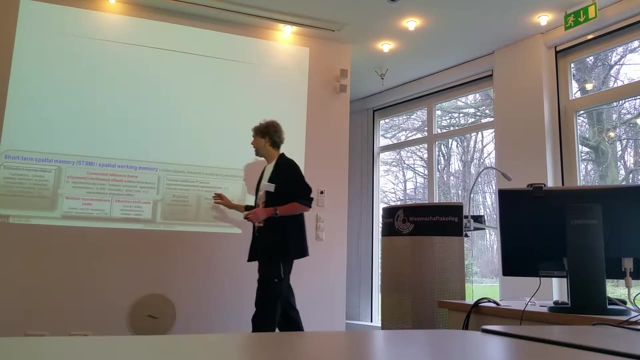 there might be a cost in just maintaining these or switching attention between these different reference frames. I think I'd like to focus on mostly here this specific conflict between two embodied representations in working memory, So concurrent reference frame conflicts. In particular. there could be two costs. 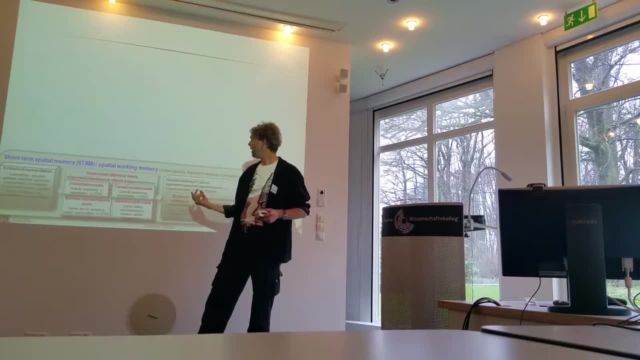 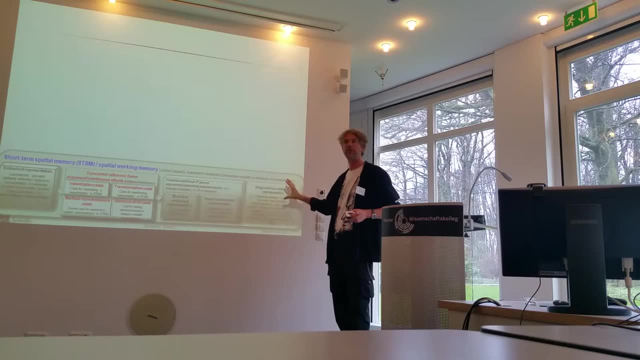 One's kind of just to instantiate an additional representation and to transform it once it's already in there. Of course you could have other representations in working memory that do not conflict, because they're not as embodied or not really that spatial. So we won't talk about this. 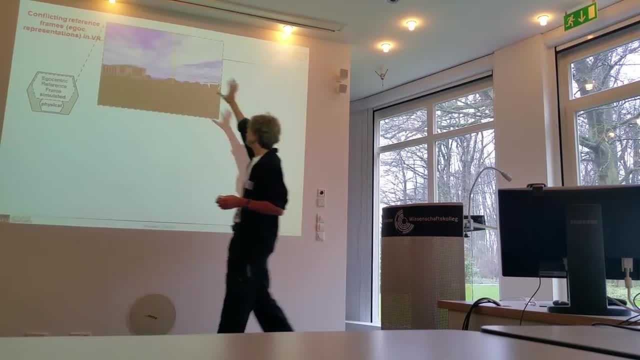 So just as an example, so if you have a simulated reference from basically what you present in virtual reality, for example, and you also have the physical environment, that is kind of the other, the physical reference frame, simply speaking, one of the reasons people like that not display so much. 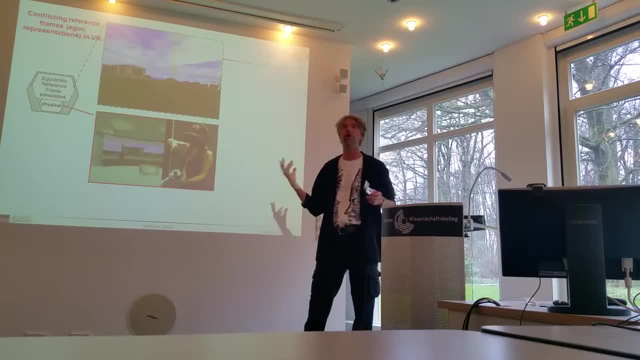 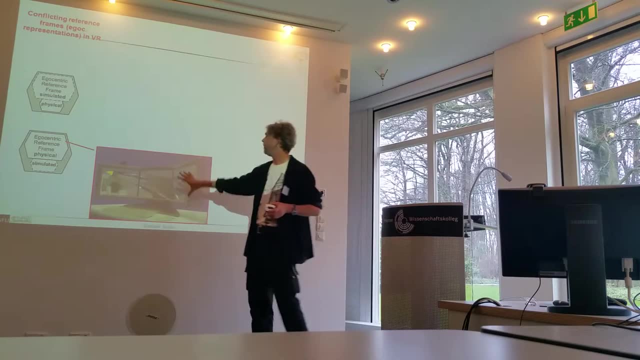 is because they basically block out your view of the physical reference frame, So supposedly you have less reference frame conflict. Another example is desktop VR, where the virtual reality is very small. so to say, you have a lot of games, so there might be more conflict. 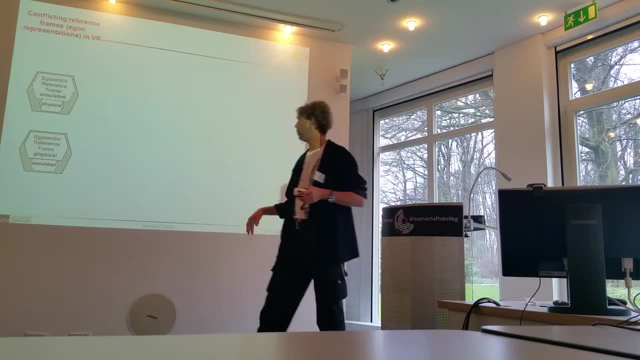 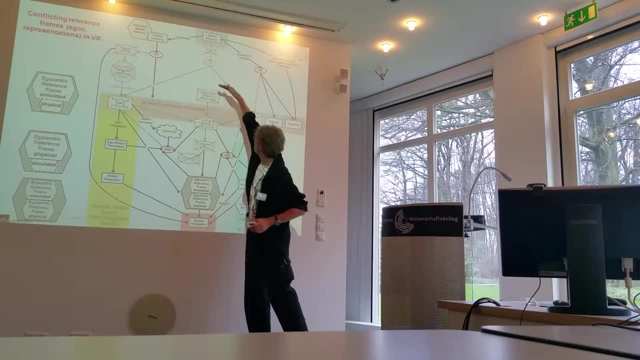 The physical might actually dominate over the simulated, or there might be more on an equal level. And in these situations where you have some kind of conflict going on in this kind of logical model, everything that's up there so dependent on this reference frame. 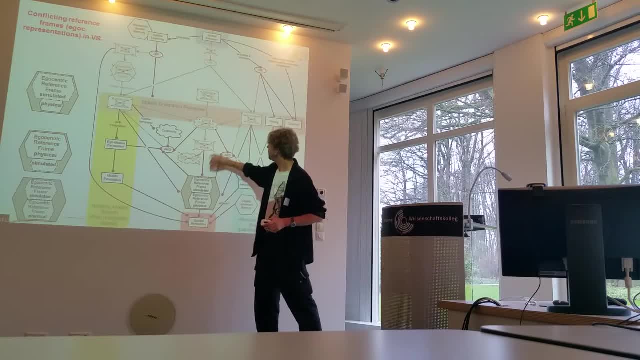 consistency will also be impaired. So there's basically interference or lack of consistency. spatial updating will be impaired and everything up there will also be impaired. So there are two automatized spatial updating processes, which are continuous and instantaneous will be impaired. 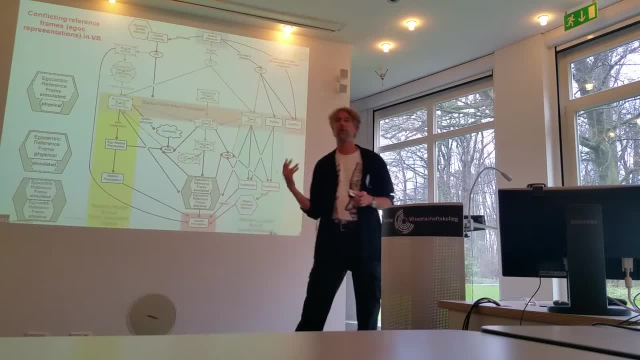 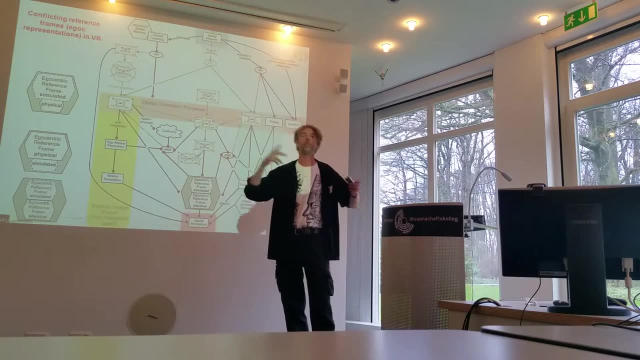 which means you will not be able to tap into these automatized, quick, intuitive processes, And we propose that. this is one of the reasons why people get lost so easily, where they hate these games, when you have to put all these landmarks into virtual environments, online gaming. 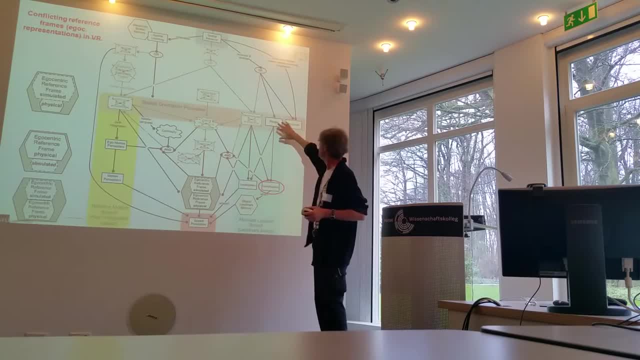 to make them work at all, Because I mean, if you can still identify them, you can do the task, and if you're highly trained and have a lot of learning, then you might still be able to do them relatively fast. but it's not that intuitive. 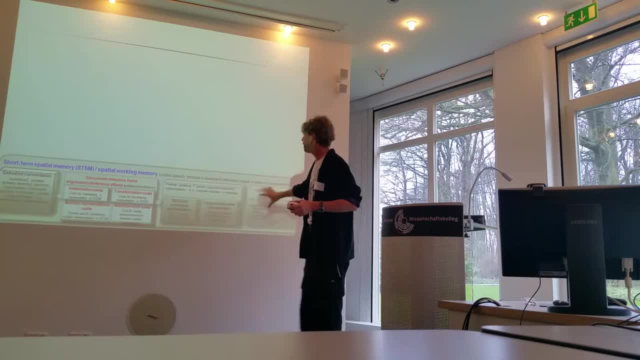 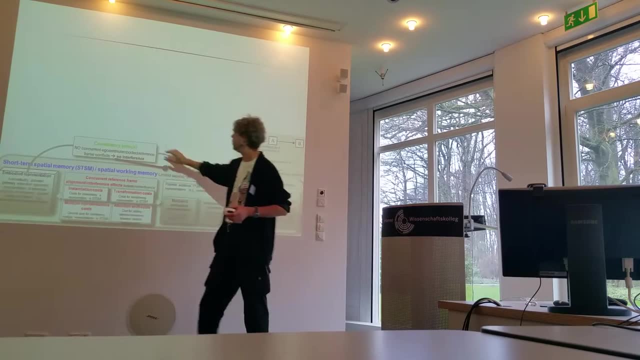 unless highly over-learned. So going back to this kind of view, just so I have a bit more space to weigh out the different parts. So if you apply this kind of idea of logic, obviously all you have to do is consistently check. 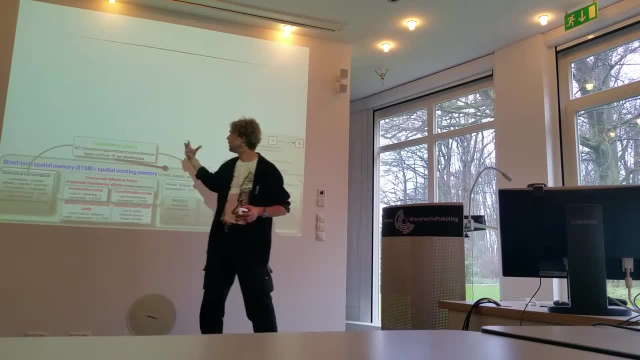 if you need spatial broken memory and it would kind of give a green light if there's no concurrent use-entry combined reference frame conflict. so no interference, And that is a necessary prerequisite for spatial presence and immersion to occur In turn. this is a necessary prerequisite. 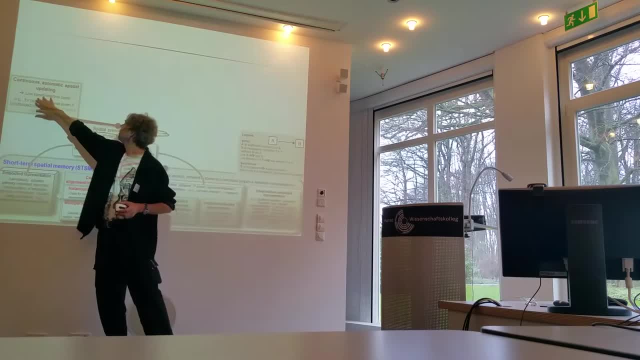 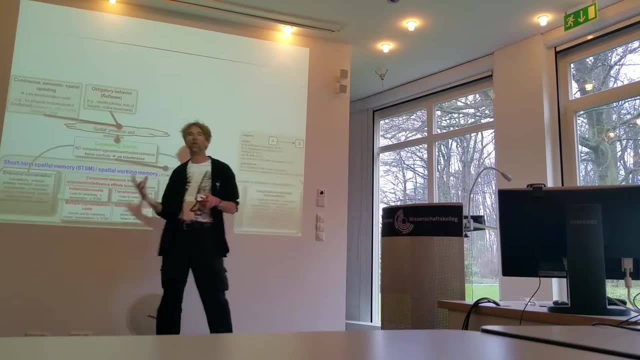 for the kind of continuous automatic spatial updating, in the sense that this allows for lower transformation costs in the air. Talking also about the fear of heights, reflexive movements, basically, only if you're fully spatially present in VR will you duck at the protein ball. 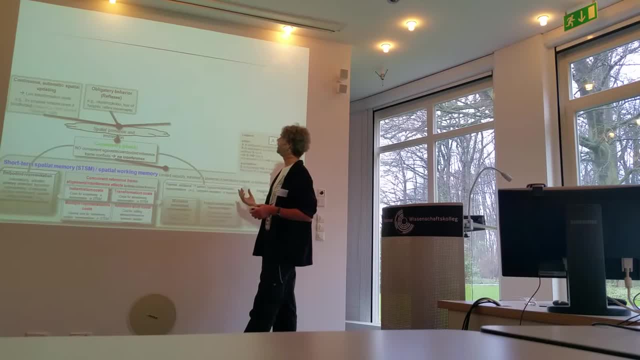 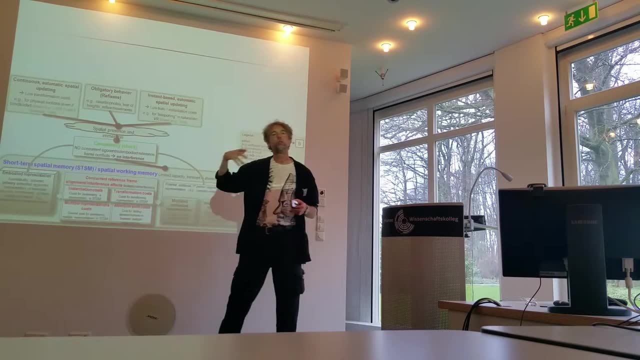 will you get fear of height, will you be experiencing interesting pit-room experiences, and so on, Similar to the instant-based spatial updating. so by being spatially present, this lowers the transformation and instantiation costs that you have with monitoring representations, And we also think that it might be necessary. 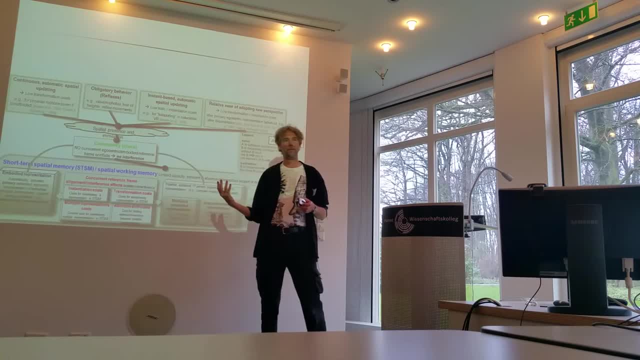 for the relative ease of adopting new perspective. So, basically, you can adopt a new perspective easily if there's no conflict with another one that you already have in memory. And now the interesting thing about logic. so there should be logic in errors. ignore that. 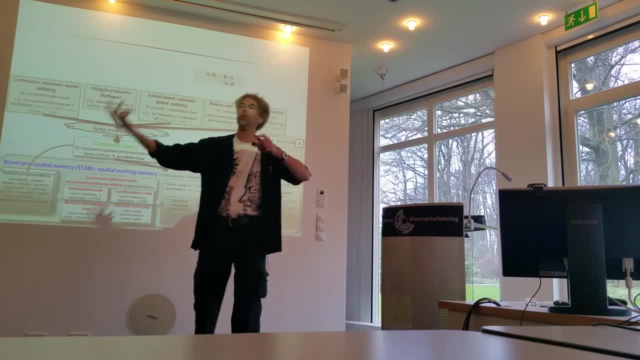 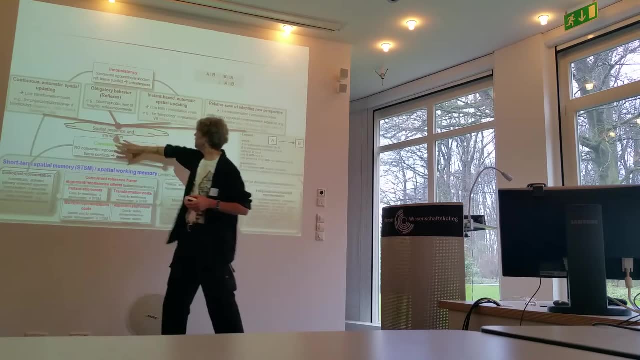 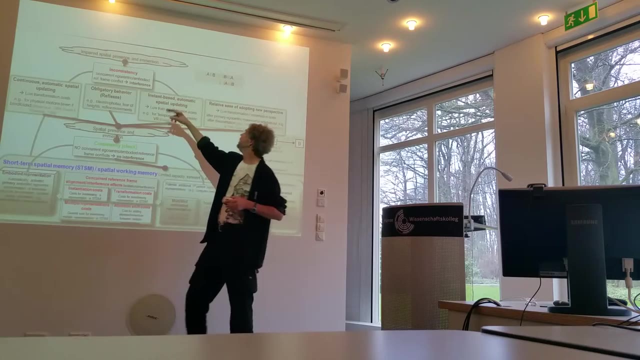 is basically if you have A implies B, you can do the math and that's equivalent to saying non-B implies non-A. So basically, if you have an inconsistency of this consistency check- so basically interference between concurrent reference frames- you kind of invert all the errors.